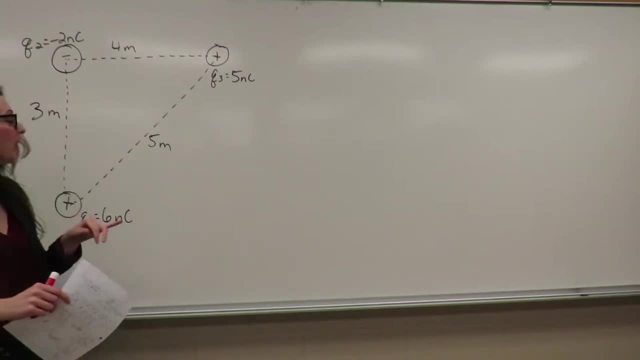 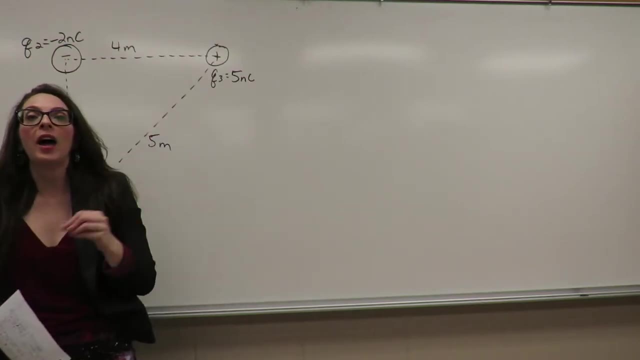 coulombs, nanos times 10 to the minus 9, and then we've got charge 2 up here with negative 2 nano coulombs and charge 3 here with 5 nano coulombs, And they're arranged on a triangle, a right angle. 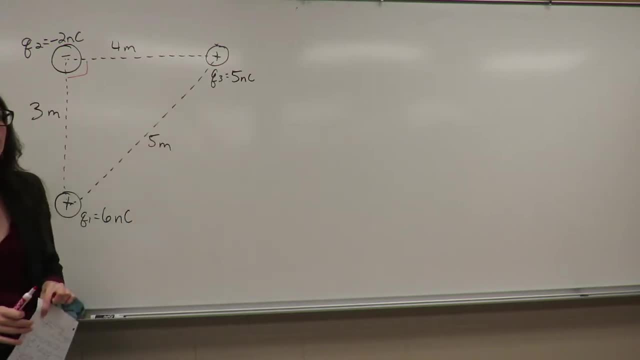 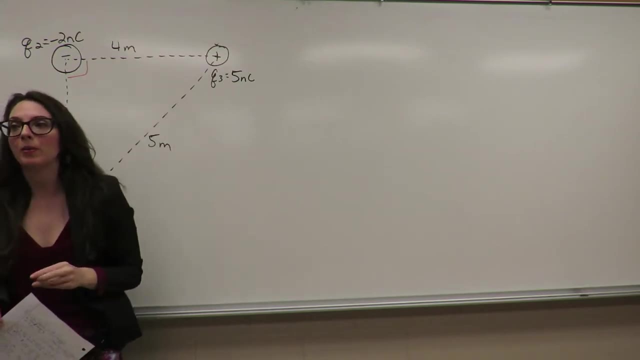 triangle, such that the hypotenuse of that triangle is 5 meters, This leg of the triangle is 4 meters and this leg of the triangle down here is 3 meters, And so the question is: we need to find the right angle triangle. We need to find the right angle triangle, So we need to find the. 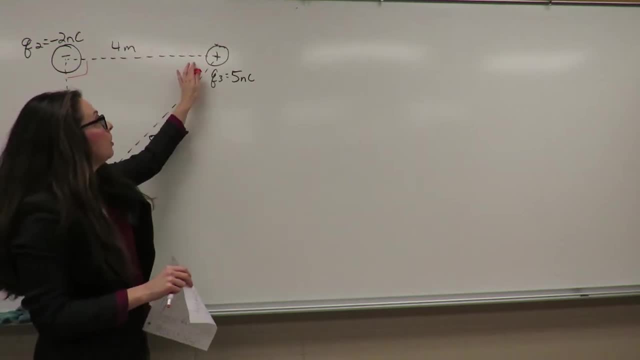 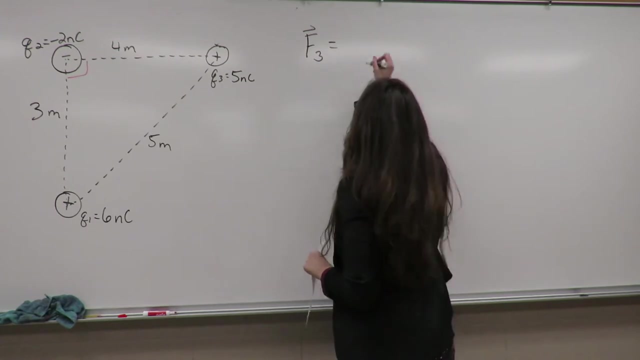 resultant force on charge Q3 from these two other charges. So what we're looking for is the resultant force F3, which is going to be equal to the sum of the force that charge 1 exerts on charge 3, plus the force that charge 2 exerts on charge 3.. 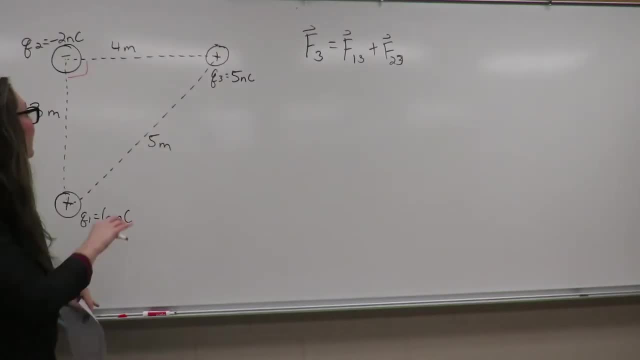 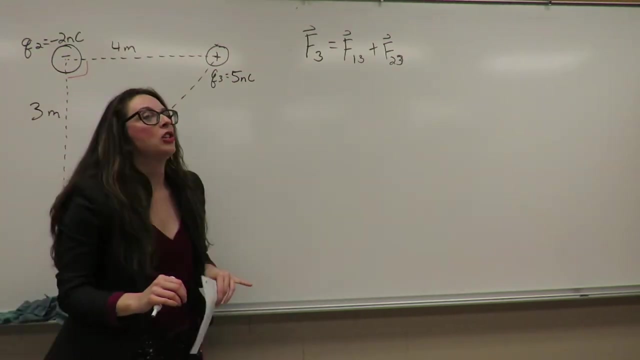 So remember that forces are vectors and in this particular problem we've got our particles, our charges, arranged in a pattern such that they have x and y components, And so we're going to have to break down this equation here for the forces acting on charge 3 here, into both the x. 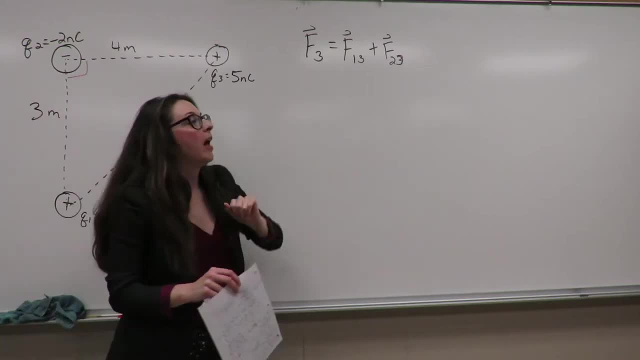 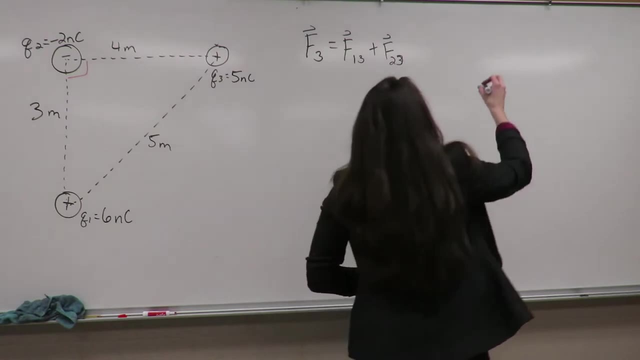 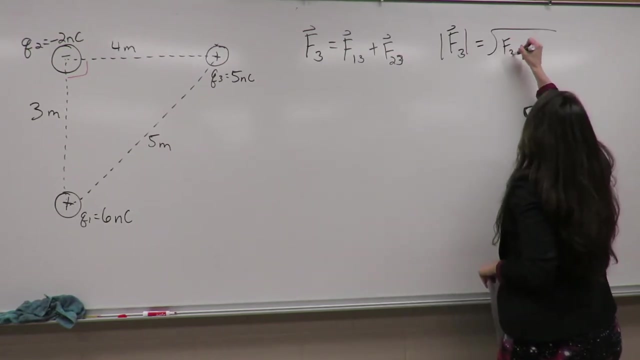 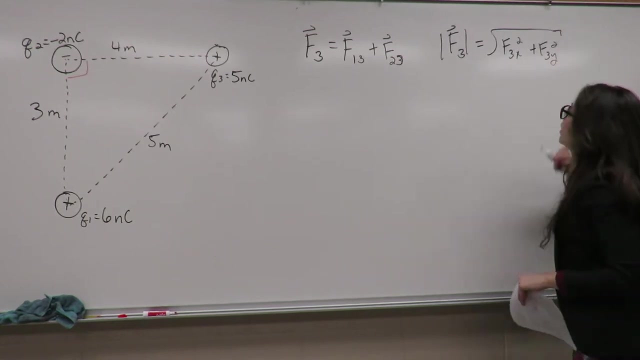 and the y components in order to in the end, get the magnitude F3 here. So remember that when we were working with vectors, we could find the magnitude of the force here, and that's the square root of the x component of the force squared plus the y component of the force squared. So what in? 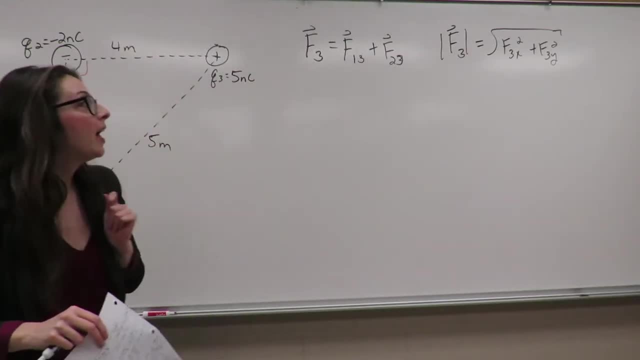 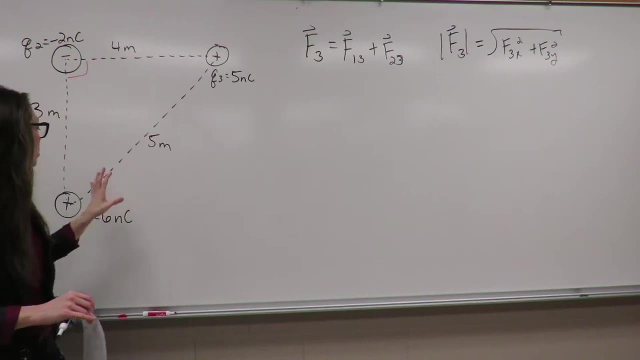 the end we're trying to get to is to get the x and y components of the force on charge 3 from charges 1 and 2.. We'll get the x and the y components and we can use them to get the magnitude of the force. 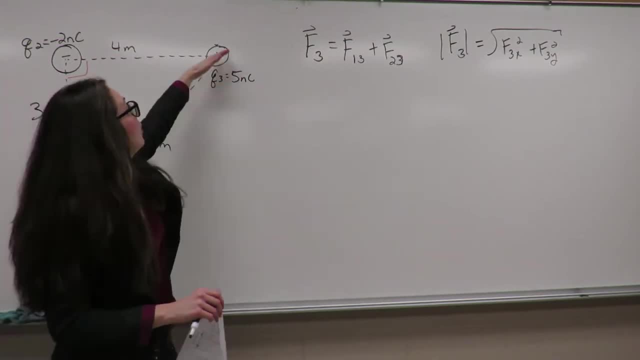 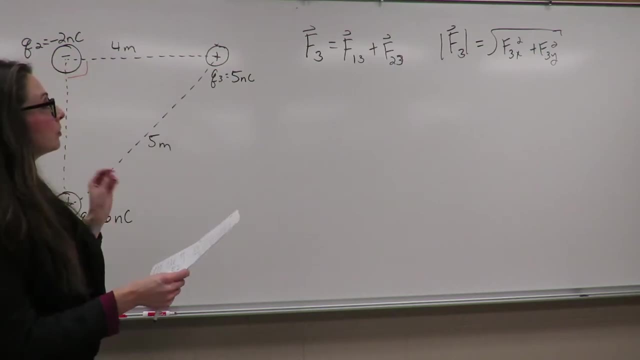 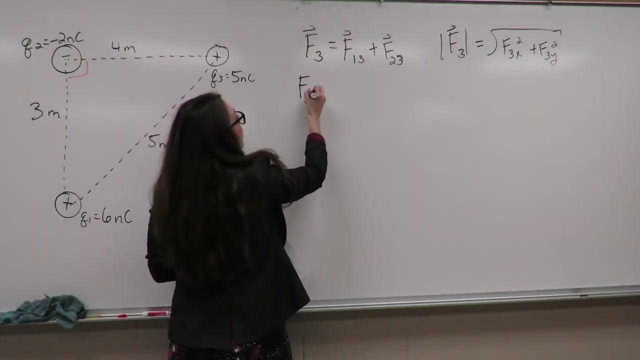 and then we'll also use them to get the angle at which this force is from the positive x-axis. So if I look at this equation, we break it up into the x and the y components, then we've got that the x component of force 3 is going to be equal to the y component of F1, or sorry, the x component. 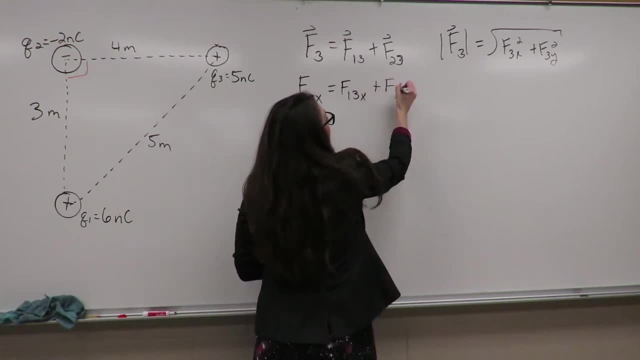 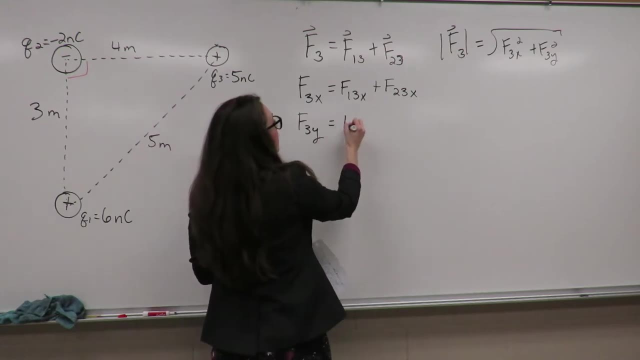 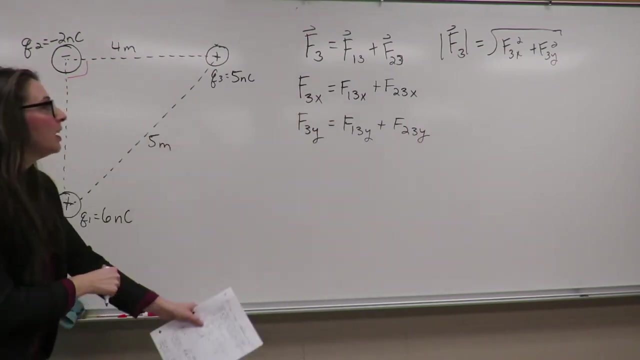 of F1 3x plus the x component of F2 3x, And then for the y portion, we've got F3y is equal to F1 3y plus F2 3y. Okay, So let's start by looking at this first component, or this charge right here. 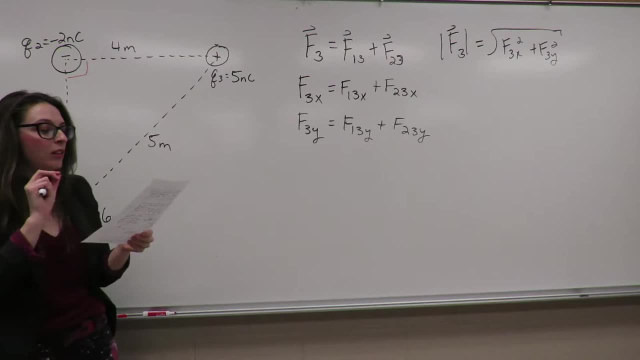 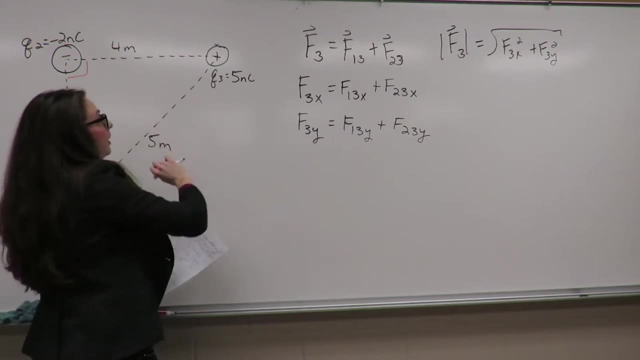 charge 2.. And so what we're going to do is find the x component of F1, 3x, and then we're going to find the force first exerted, the force that Q2 exerts on Q3.. So the force exerted by Q2 on Q3.. 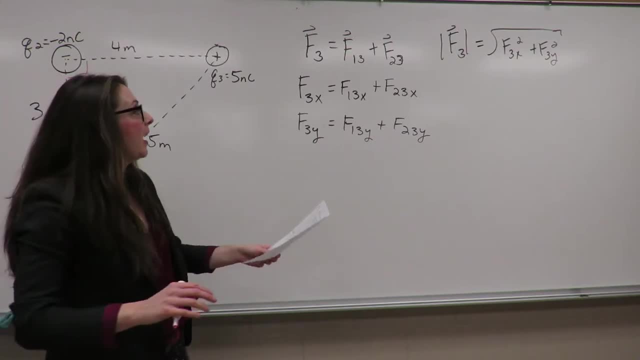 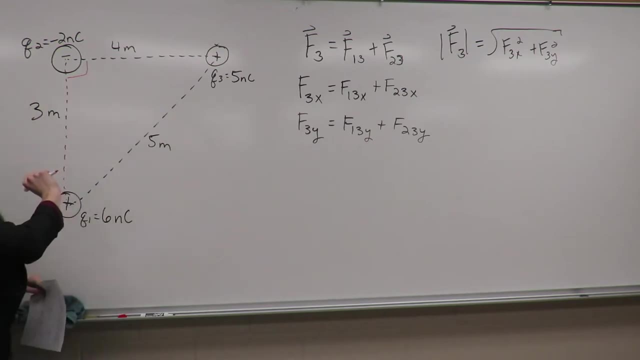 And actually, if I go ahead and draw what that vector looks like, the vector F2- 3,- well, let's see We've got a negative charge for Q2, a positive charge for Q3.. Those are opposite charges. so 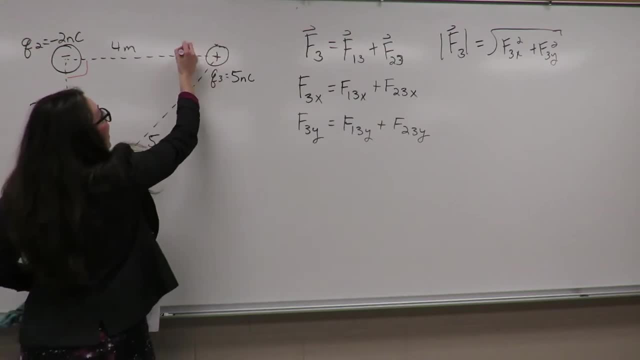 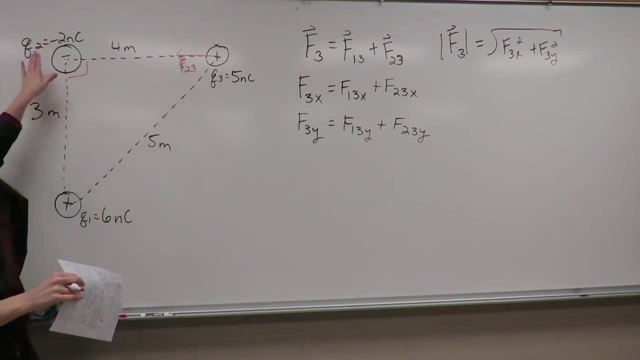 they're going to be attractive for Q3.. So we're going to find the x component of F1 3x and then we're going to find the force. So if we draw F2 3, F2 3 here is going to be pointing toward directly charged Q2.. 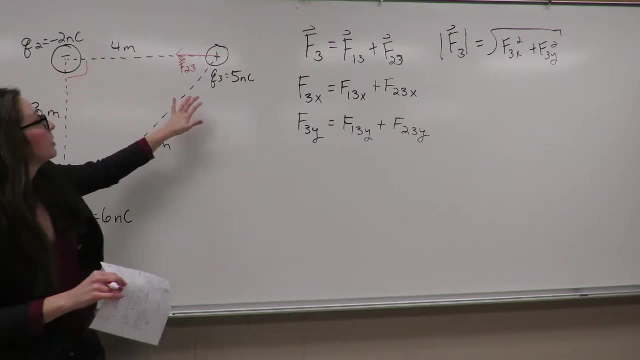 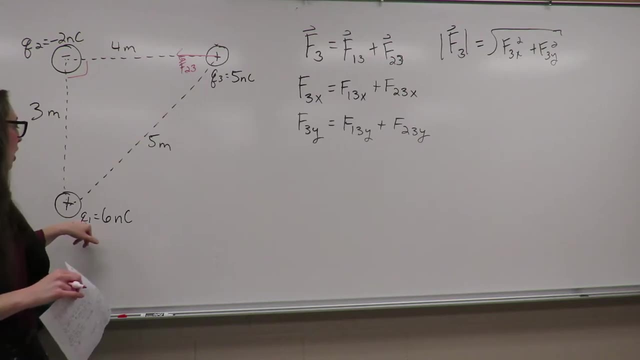 So the force that Q2 exerts on Q3 is going to be pointing directly toward Q2.. Now for our positive charge, Q1, the force that Q1 exerts on Q3, if we draw that vector, well we've got. 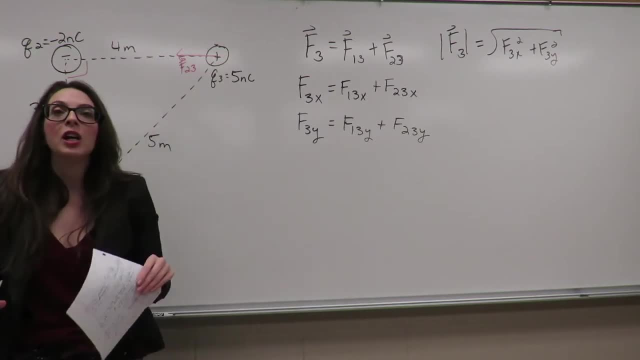 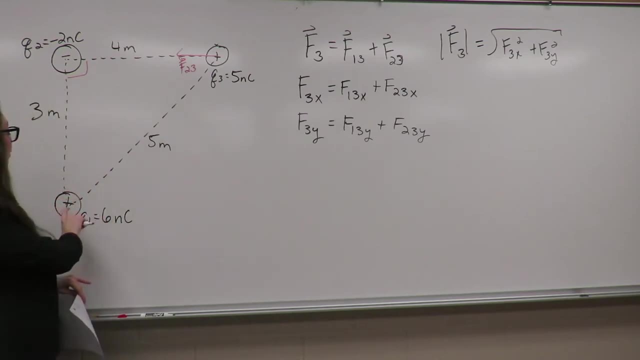 Q1 is a positive charge. Q3 is a positive charge. Like charges repel, and so the charge, sorry, the force that Q1 exerts on Q3 is going to be pointing in the opposite direction of Q1 here. So it's going to be. 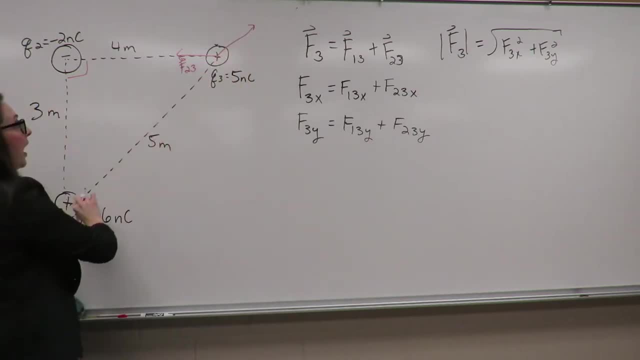 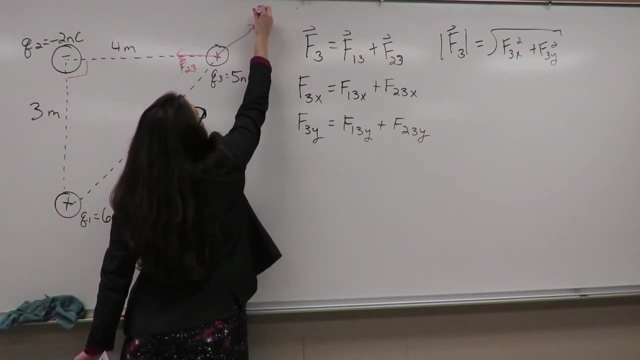 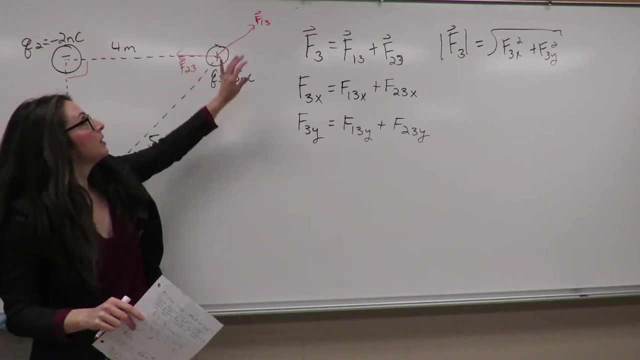 pointing directly off along this line, along the hypotenuse. It's going to be pointing off up here in this direction. This is the force F1- 3x That charge 1 exerts on charge 3.. Okay, so that's what these components of the vectors look, or that's what 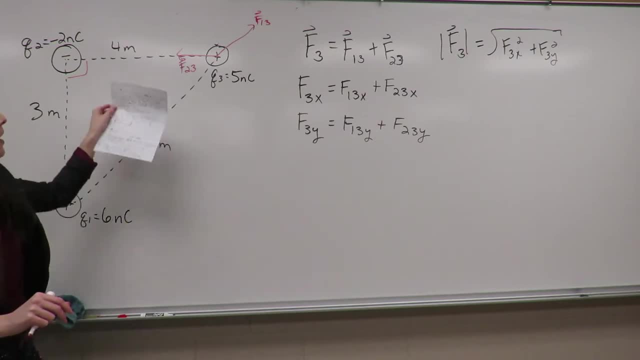 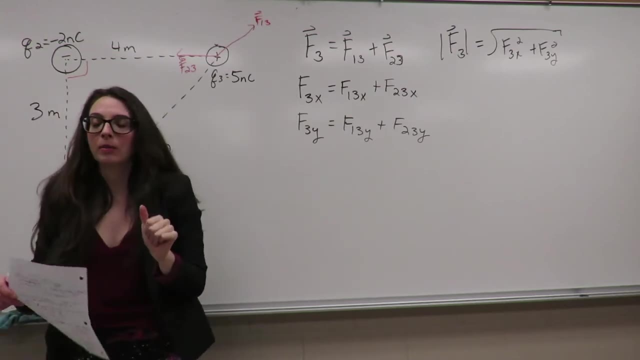 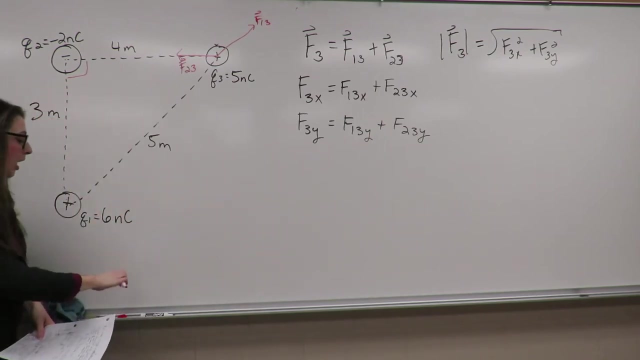 these vectors individually look like and we need to break down F2- 3 and F1- 3 into both their x and the y components so we can stick them in this equation, right here, in these two equations. So now let's start back with finding the components of the force F1- 3x. 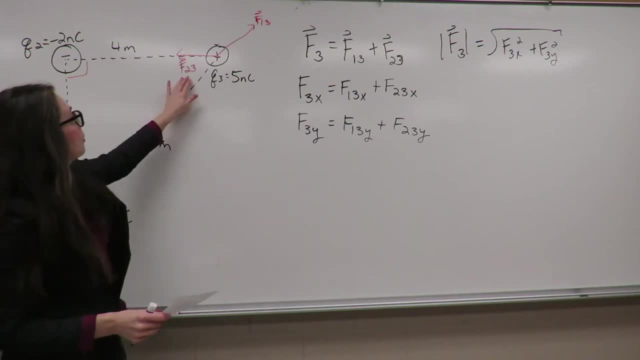 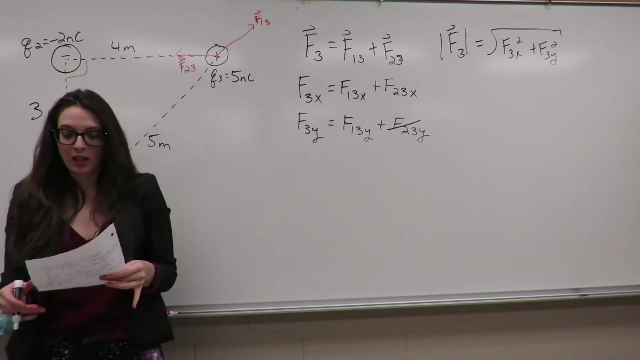 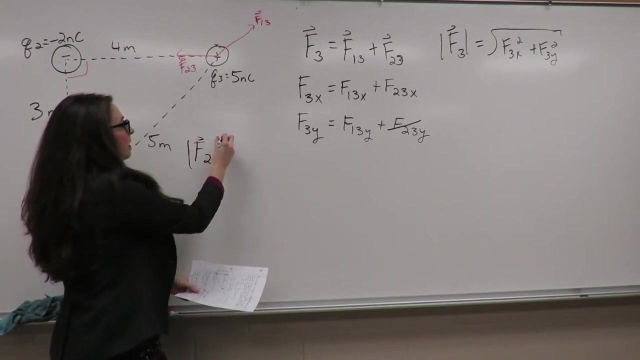 Okay. so if we look here, F2 3 is only in the x-direction. There's no component of F2 3 in the y-direction, and so I can just actually go ahead and cross this out of my F3y equation here. Now, the magnitude of F2 3 is going to be equal to the Coulomb constant K. 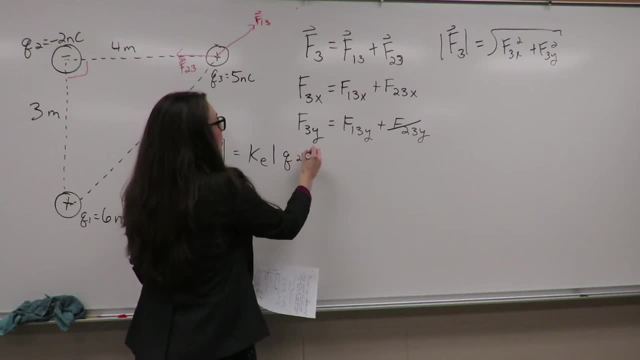 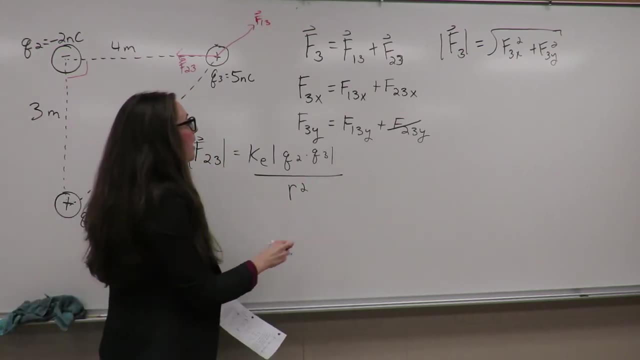 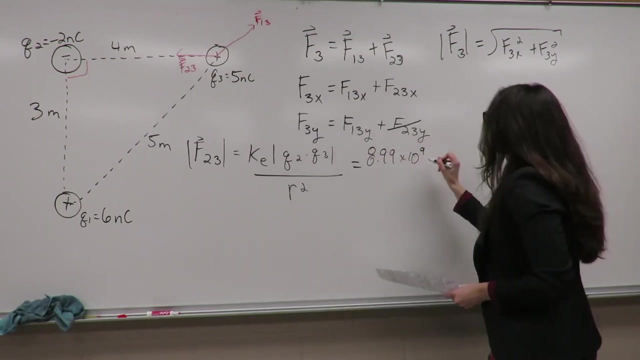 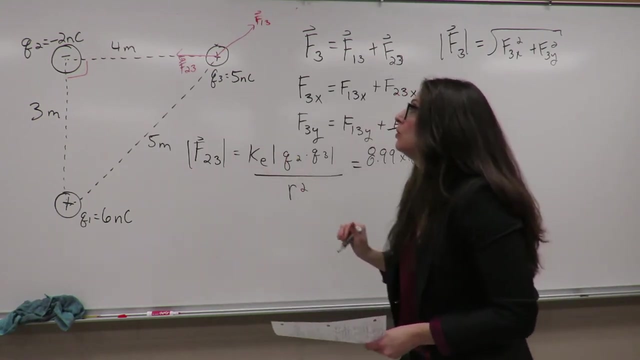 Okay, times the absolute value of Q2 times Q3, all over the distance between them squared. Okay. so this is going to be equal to 8.99 times 10 to the 9 Newton meter squared over Coulomb squared, times the absolute value of charge, Q2, two. 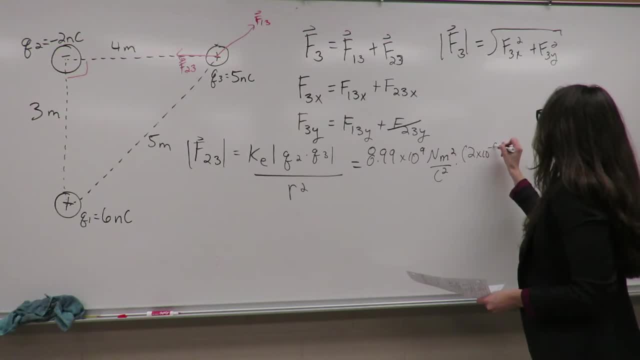 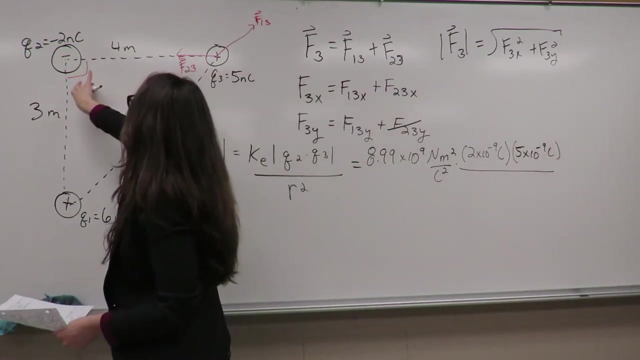 nanocoulombs. So it's going to be 2 times 10 to the minus 9 Coulombs, Times our Q3 5 times 10 to the minus 9 Coulombs, And then we're going to divide that by the distance between them. squared, The distance between Q2 and Q3 is 4 meters. 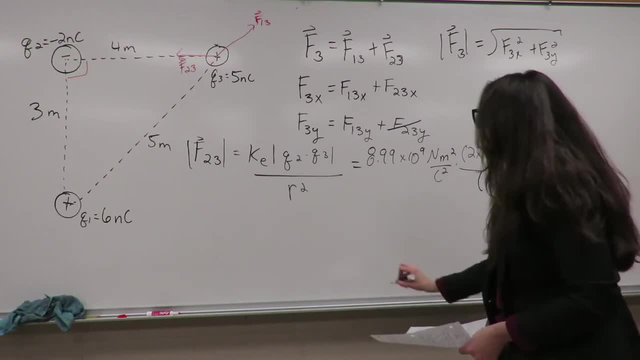 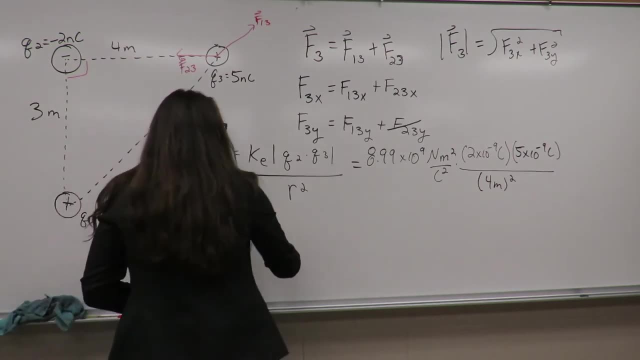 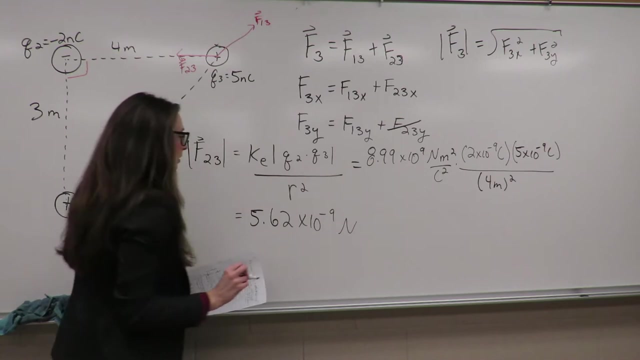 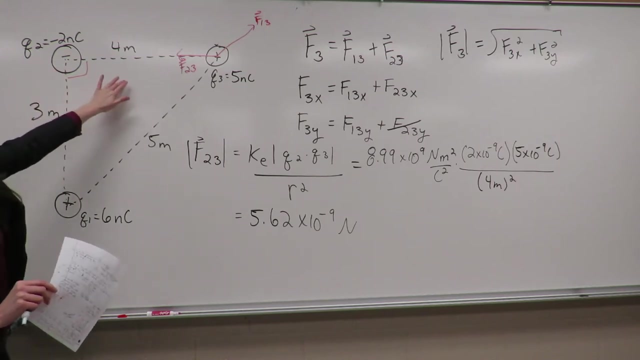 So divide that by 4 meters squared, Okay, so plugging those into my calculator, I get that the magnitude of F2: 3 is going to be equal to 5.62 Newton meters squared over C2.. times 10 to the minus 9 newtons, So that's the magnitude of F23.. Now, since F23 only. 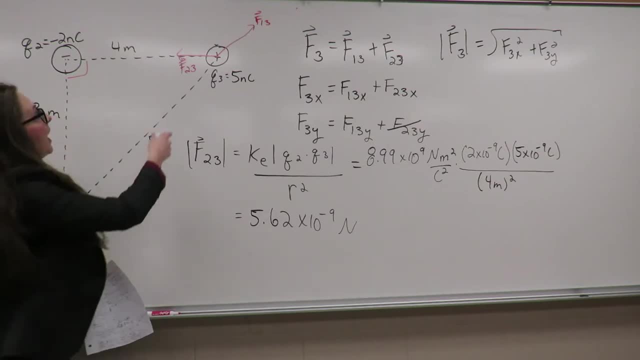 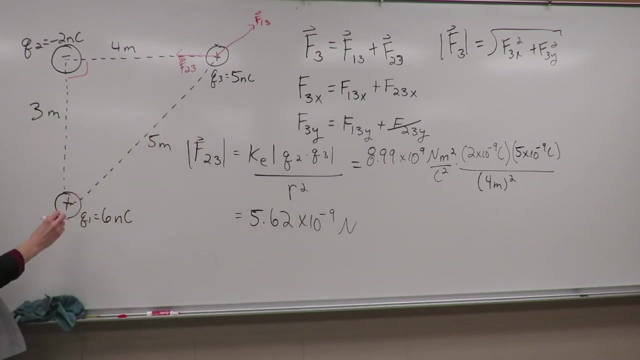 has a component in the x-direction and since that x-direction was pointing, or that vector is pointing, in the negative x-direction, then I have that my force. let's see where am I going to write this. I have that my force. F23. 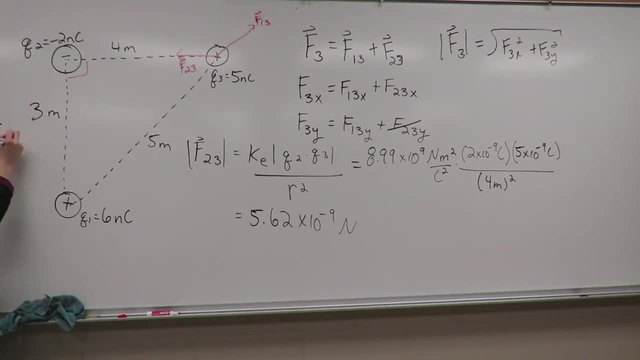 x is equal to 5.62 times 10 to the minus 9 newtons. And then there's no component of, there's no y component of F2y, That's just zero. So I'm sorry, F23y is just zero newtons. Okay, So now that one was the easy one. Now let's work. 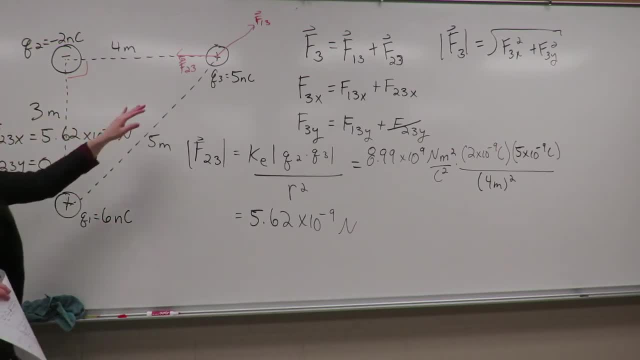 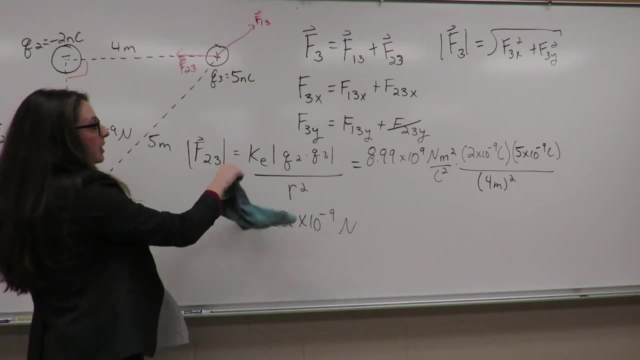 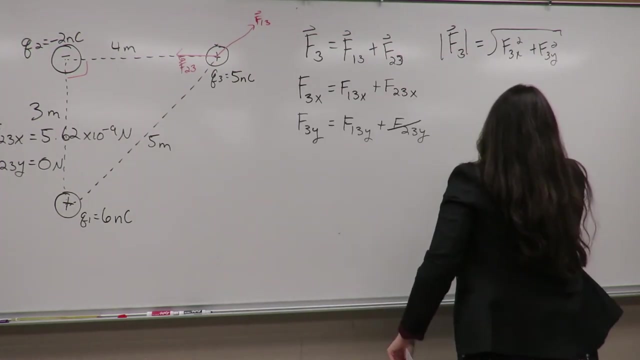 together. I'm finding the components, the x and y components of F13. So I'm going to go ahead and erase what I did just right here. Now, as you can see by this vector here, F13 has both an x and a y component. So if I go ahead and draw in, 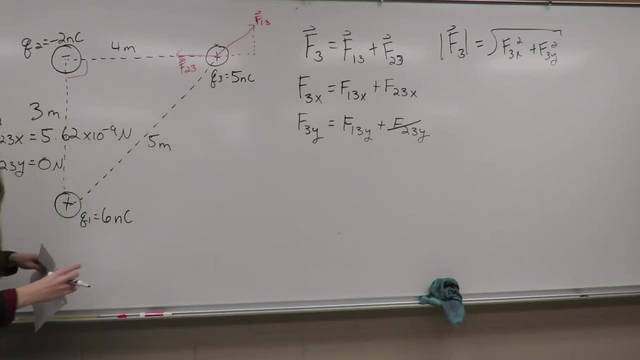 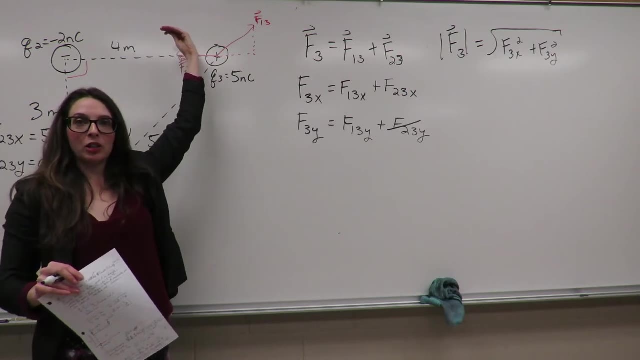 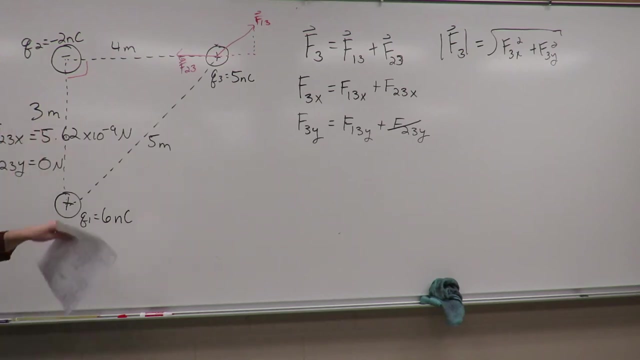 those look like here. Oh, and one thing I forgot. So we're back on the x-direction. So back over here we were talking about F23x. F23 is pointing in the negative x-direction toward Q2.. So F23x actually has a negative sign there. It's negative 5.62. 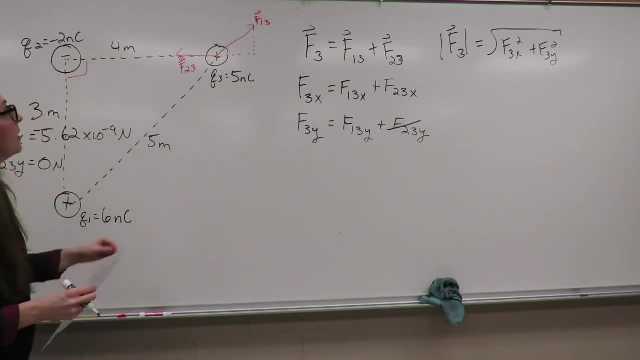 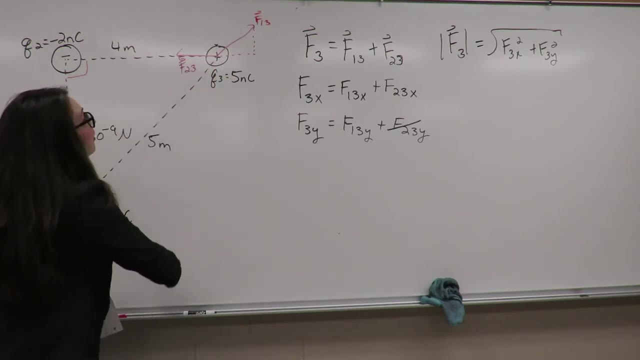 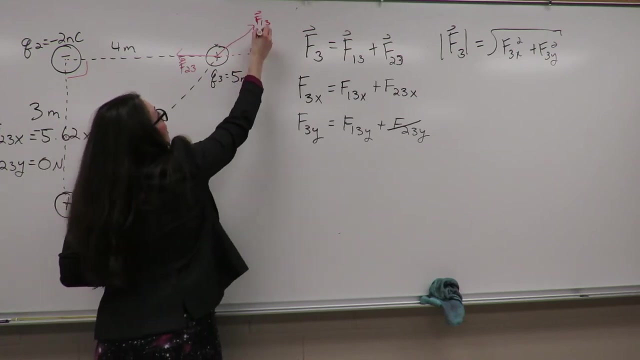 times 10 to the minus 9 newtons. Alright, so now we are going to work on F13. And so we can see here: this is my F13 vector and it has an x component or a y component, right here, F13y, has an x component, right here, F13x, And there's. 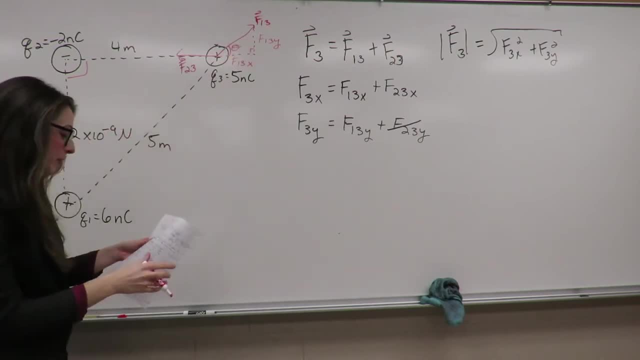 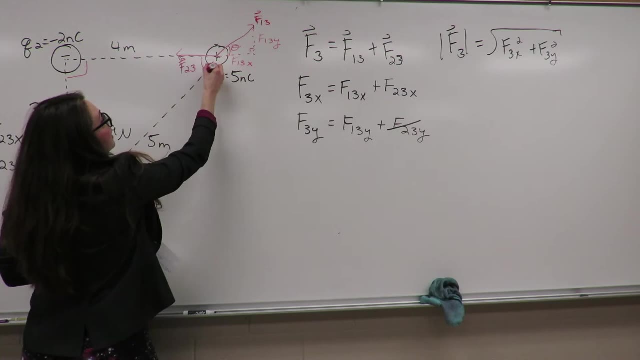 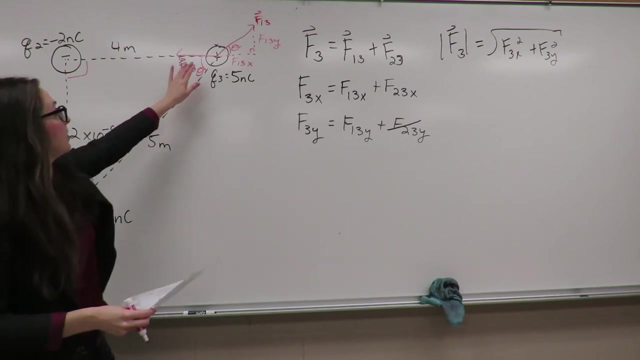 some angle in here. We're going to call that angle theta, And this angle here theta is also the same as this angle inside the triangle. We're going to call that angle theta as well, And so this comes from geometry, the reason why these. 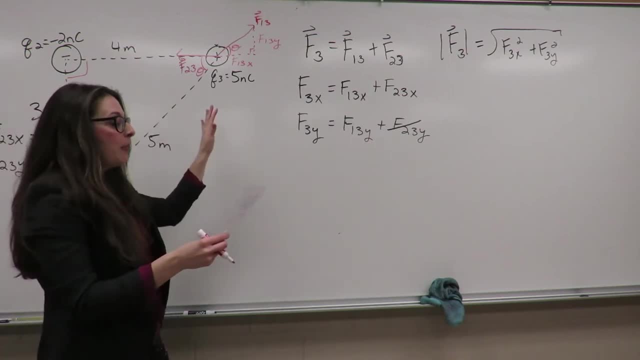 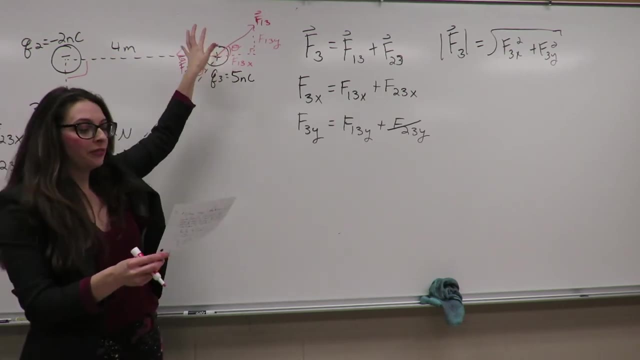 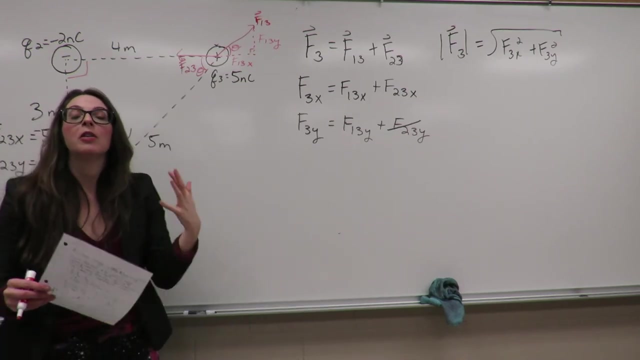 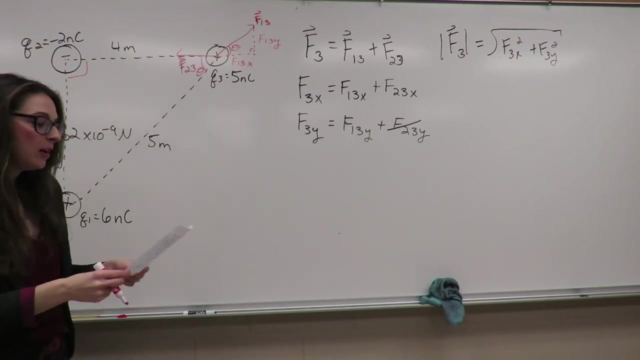 two angles are equal, Angles opposite each other. when two lines cross, those angles are equal with each other. These angles are called vertical angles because they share the same vertex. Vertical angles because of the sharing up the same vertex. Okay, so we've got that figured out right there. 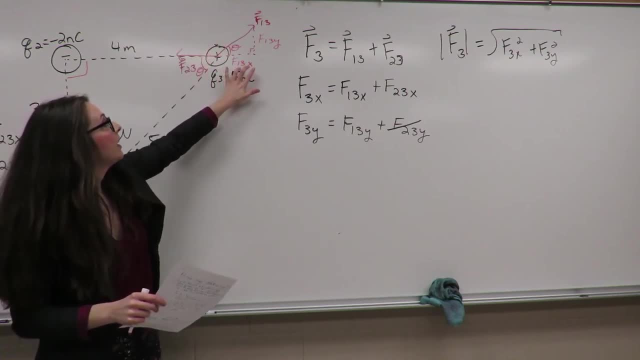 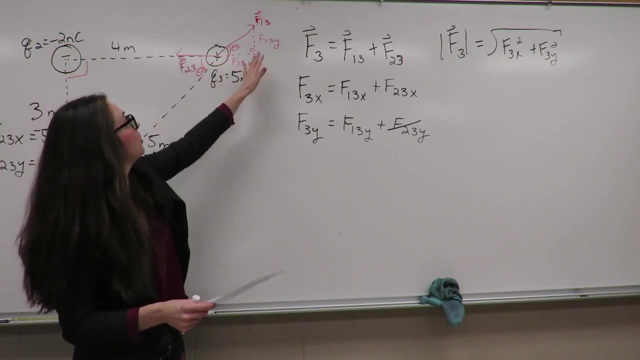 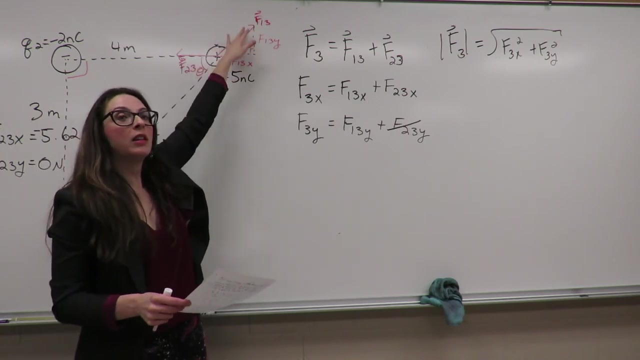 So we've drawn it out. We see that there's an x and a y component of f. But before we move forward too much with getting their x and y components first, we need to get the magnitude of what this vector is essentially. the 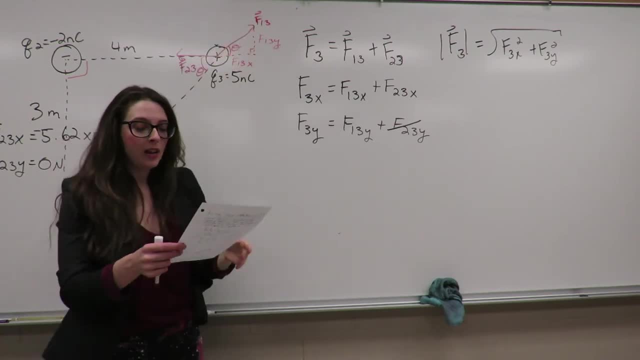 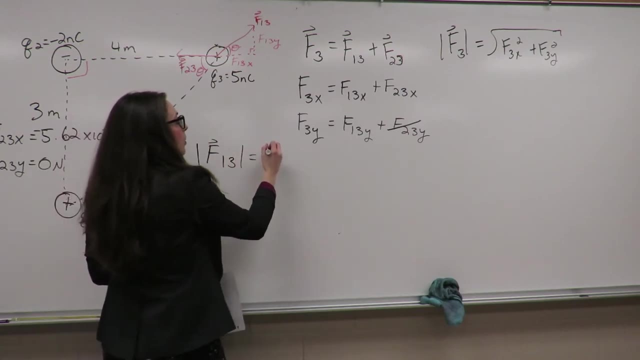 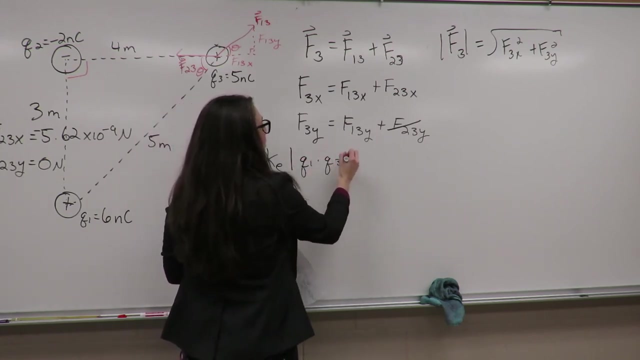 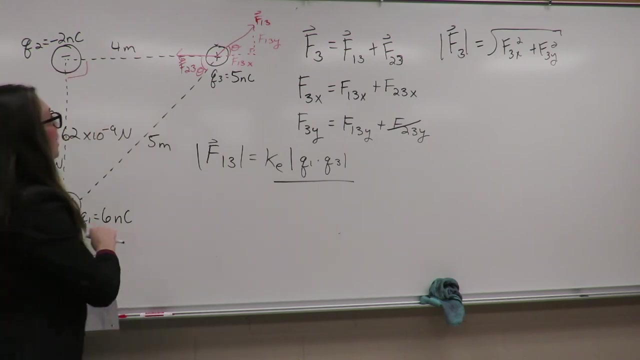 magnitude of this hypotenuse, of this little triangle that we just drew right here. So the magnitude of F is going to equal to our Coulomb constant K times the absolute value of Q times Q, all over the distance between them squared. Okay, and so the distance between: well, we'll get to that. 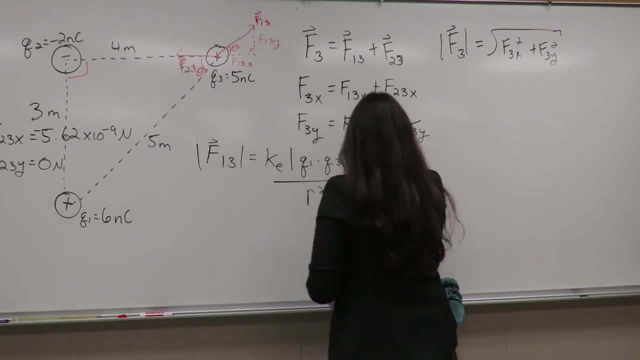 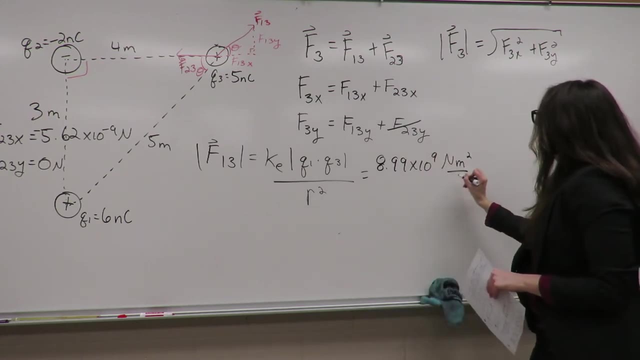 the distance between them squared. Okay, and so this is going to equal to 8.99 times 10, the 9. M classified by Coulomb squared times the absolute value of charge, one which is 6 times 10 to the minus nine Coulombs. 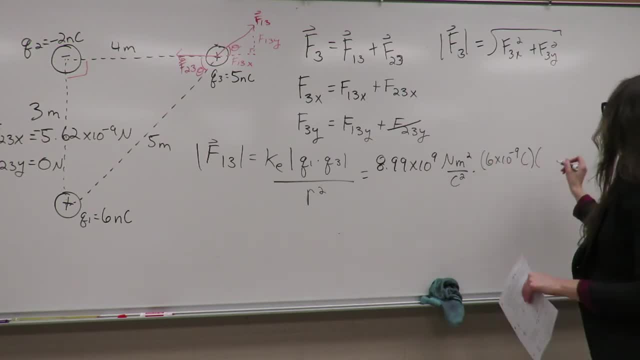 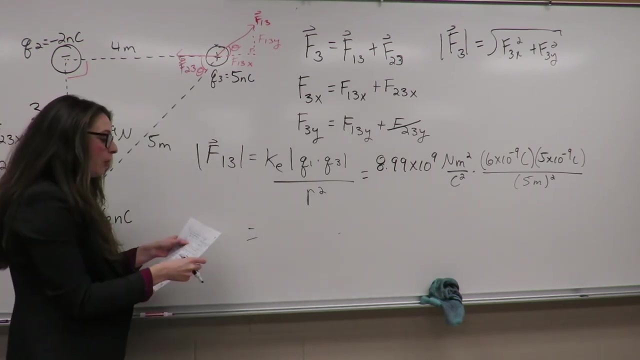 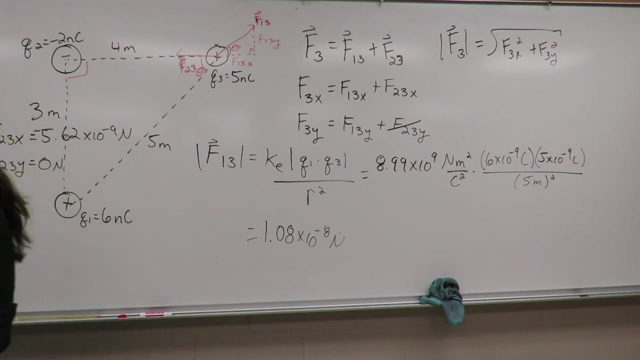 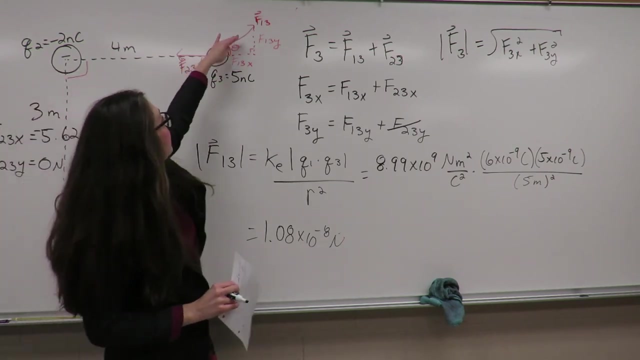 times our charge, three, 5 times 10 to the minus nine Coulombs divided by the distance between them squared, So five meters squared. If I plug those in to my calculator, I get that the magnitude of F 1.03 is 1.08 times 10 to the minus 8 newtons. Okay, now that's the magnitude, right here. 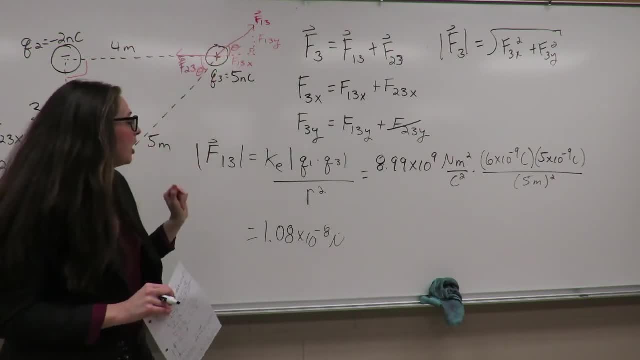 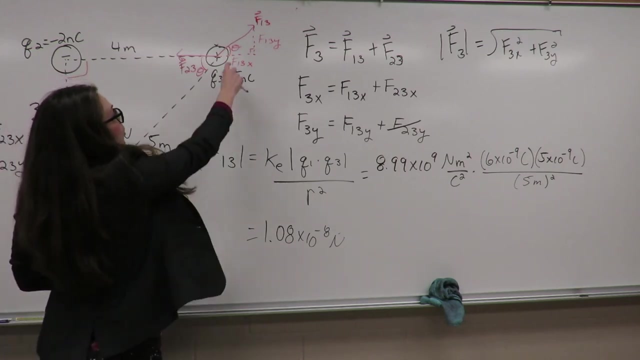 essentially this hypotenuse of this triangle there, and we need to get the x and the y components now of this vector. So, in order to do that, one thing that we also need to know is: what is this angle theta? right inside here, It's actually up here. I'm going to write that the 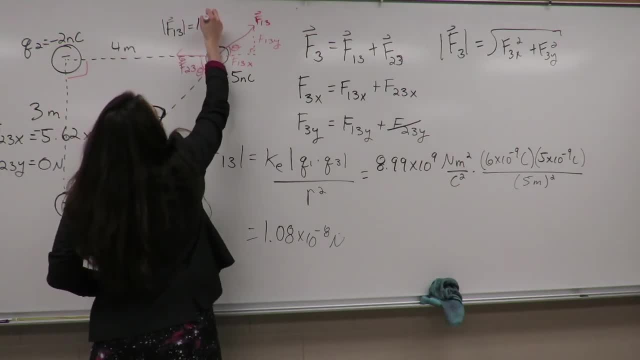 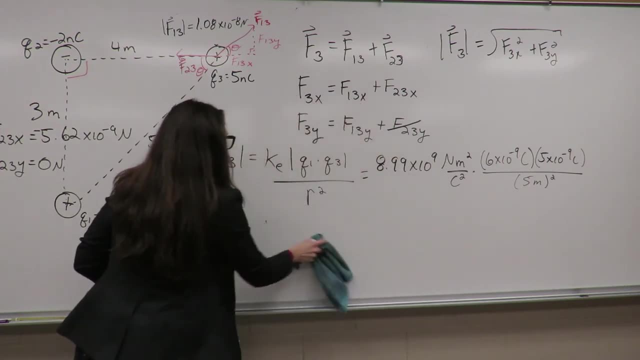 magnitude of F13 is equal to 1.08 times 10, to the minus 8 newtons. so I can erase all of this right here. Okay,